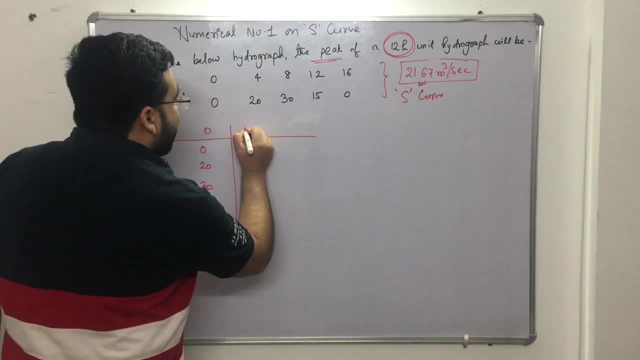 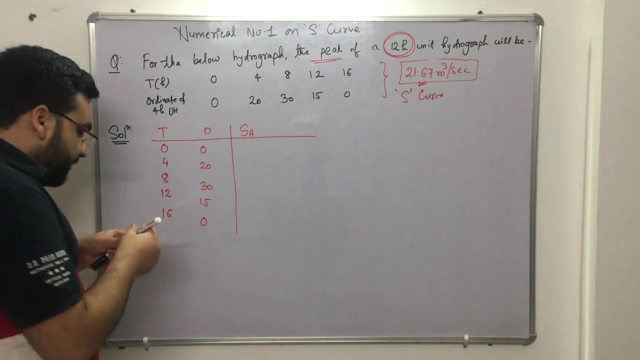 us make an S curve, right? so first of all, let us make a S curve and denote it with SA. SA is the first S curve. so how to get the S curve? so, if you remember, let me take another marker. so if you remember, yeah, this marker. so let, if you remember, 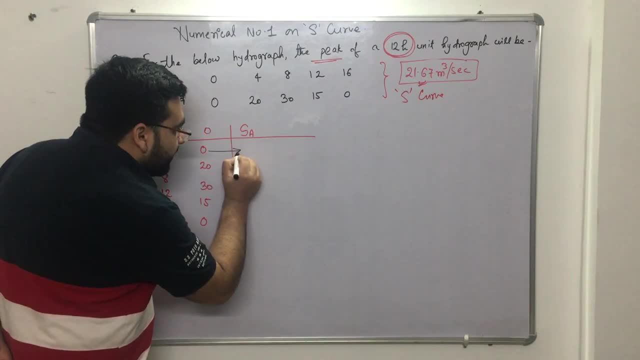 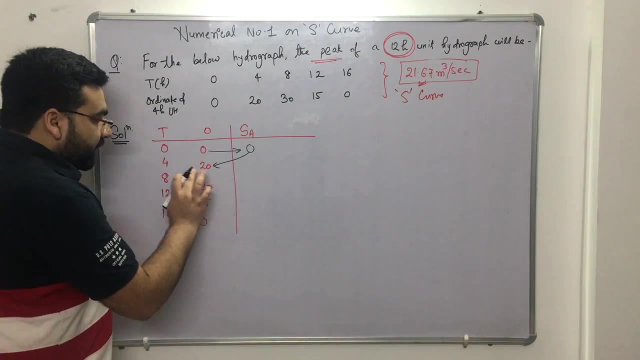 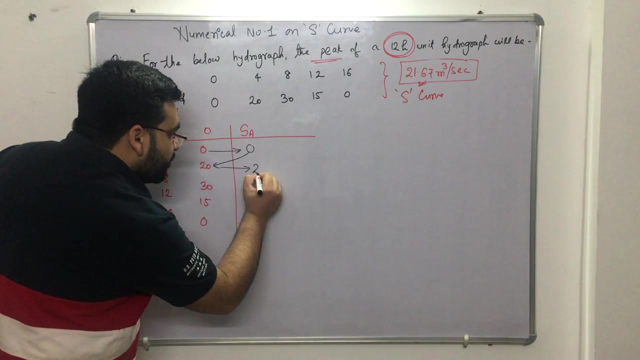 so we have to. we have to write directly like this: this is 0. okay, now, we have to take this to this point, right. so this is 4 plus we have to take this to this point, right. so 20 plus 0 will be equal to 20. yeah, now we have to take to this. 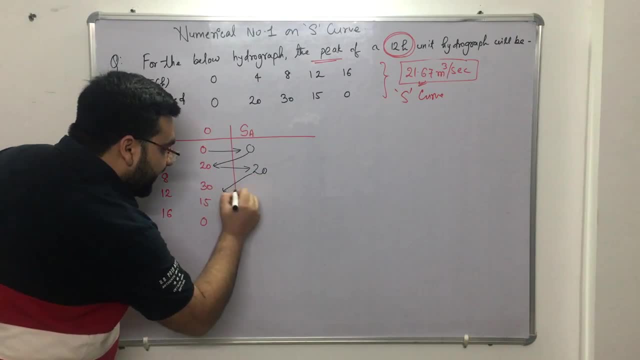 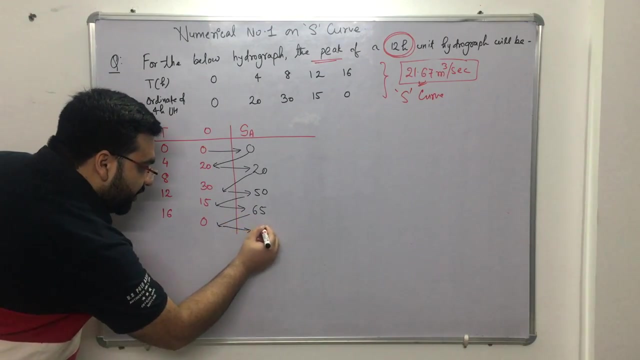 point: right now: 20 plus 30, that is, yeah, now 50 to this point: 50 plus 15, that is equals to 65 right now. then here also: 65 plus 0 is 65, and soon you will be getting 65. only this is step number one. 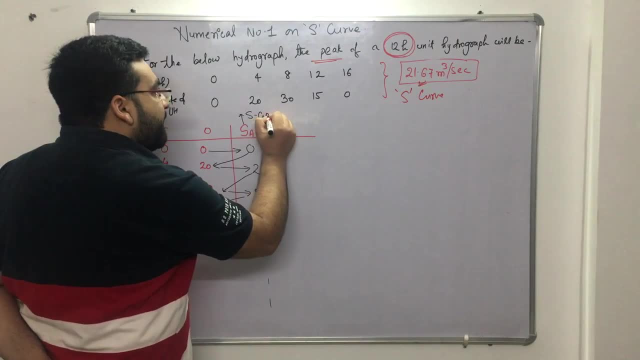 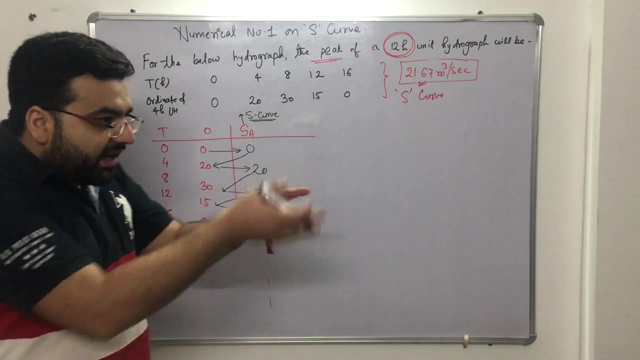 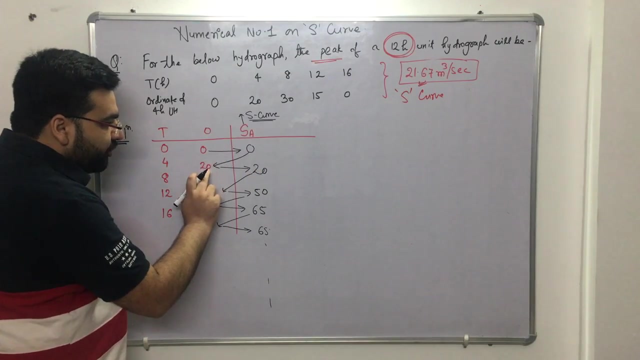 to get the S curve. now we have got the S curve. so I am talking about, I am solving the steps, the steps which you have right. this you could also do by using a lengthy calculation, but then will be very lengthy. so this is a short technique which I have already told you. so take it here: 0, 0 plus 20, so much, or you can do. 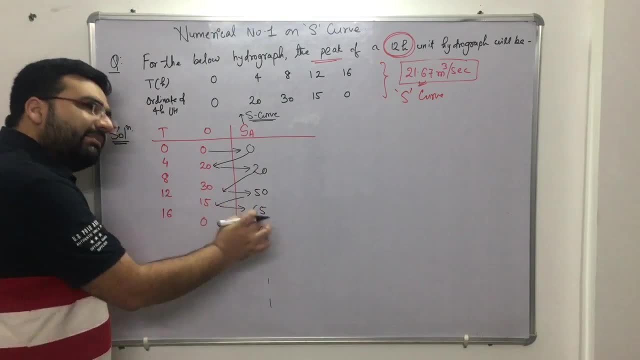 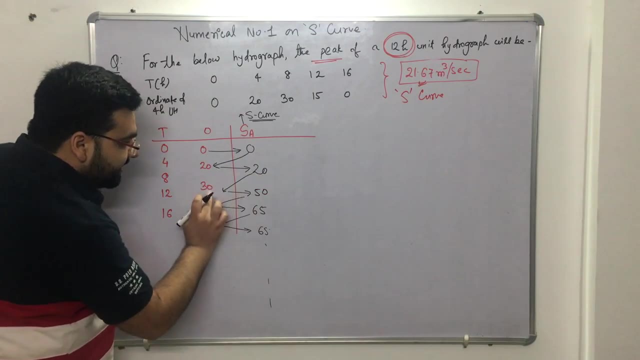 it like this: lag by 0, 20, 30 and do the same thing. that will also, so you will get the same answer, but to again make the step shorter, so 0, 0 plus 20,, 20,, 20 plus 30,, 50,, 50 plus 15, 65, 65 plus 0,, 65 plus 0, 0, 0, and so on. 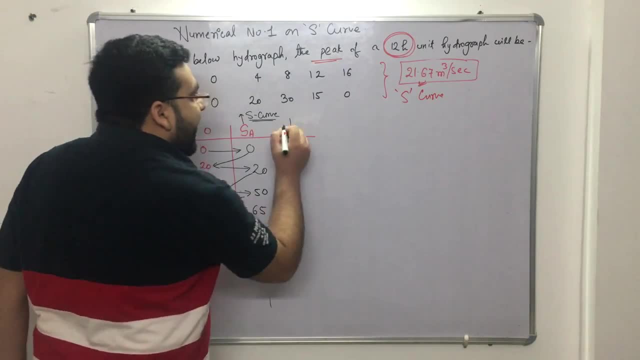 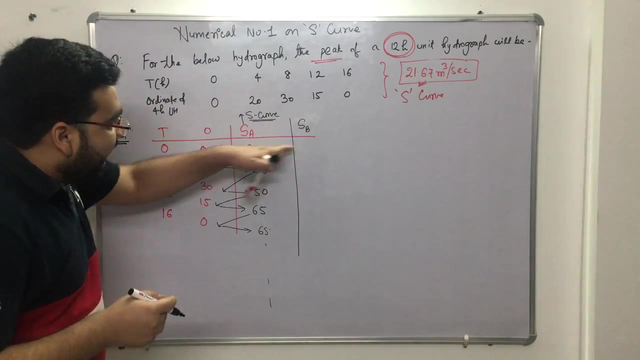 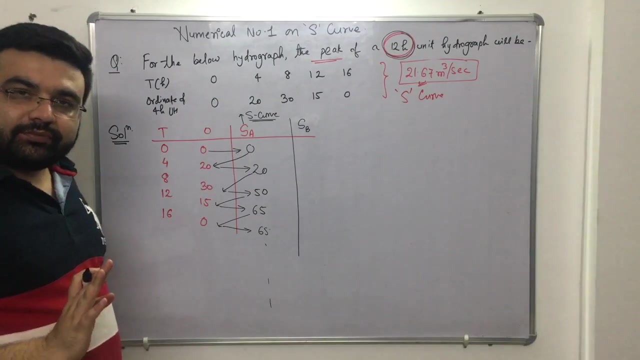 Now step number 2, if you remember. now step number 2 is I have to make another S curve, which I denoted with SB in SB. what I have to do, I have to lag this S curve with how much of amount? whatever is asked in question, that is by TRs clear. 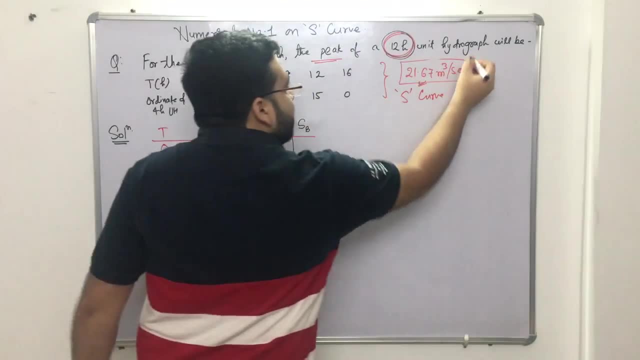 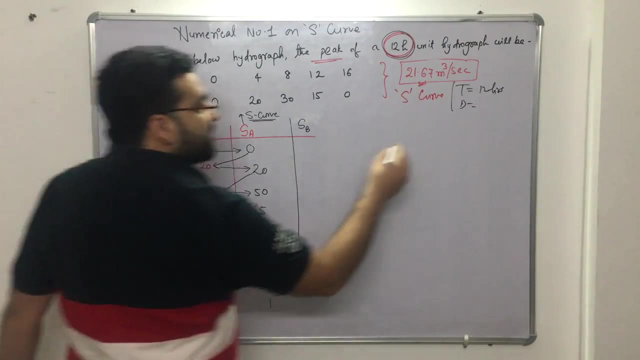 So how much is T? So T is 12 hours. let me write here: so T is 12 hours and D is how much D is 4 hours. so 4 hours. you don't have to work 4 hours clear. 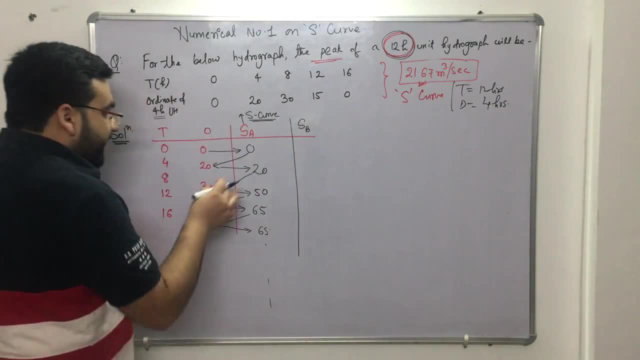 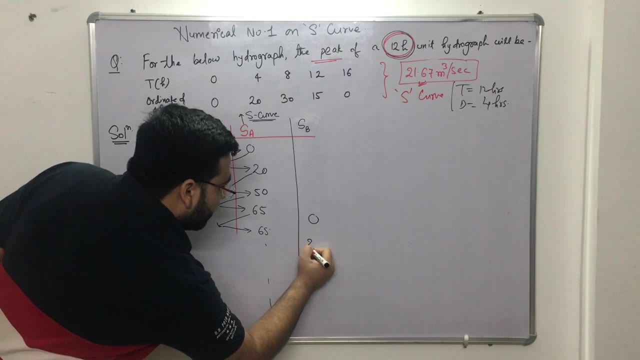 Now SB. so I have to lag it with 12 hours right. So 0,, 4,, 8,, 12, so it will start from here. So is it clear. So this is 0, right Now. this will be 20, clear. 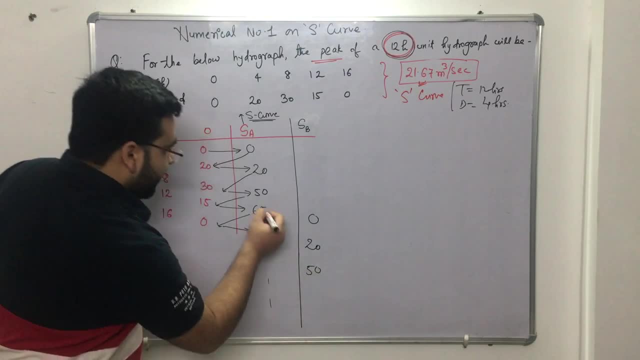 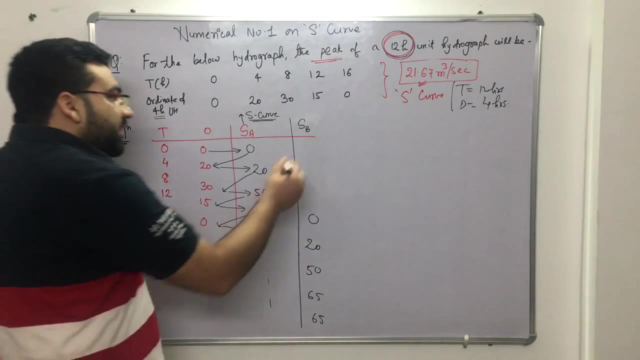 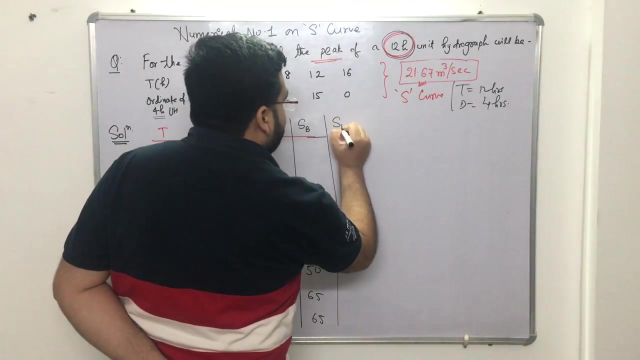 20,, now it will be 50,, now it will be 65, now again it will be 65, and so on. clear, Now the third step, if you remember, third step, we have to do SA minus, SB, SA minus. 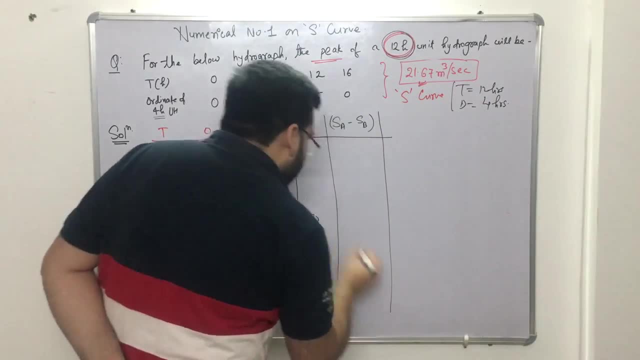 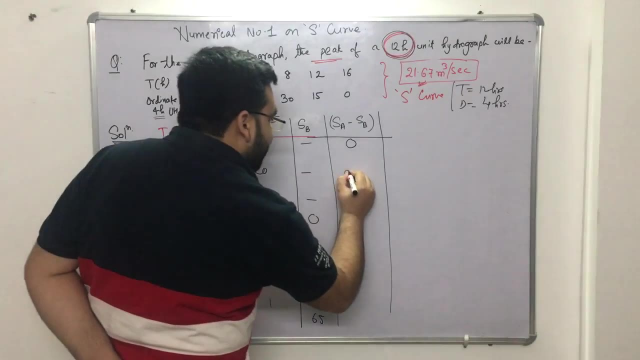 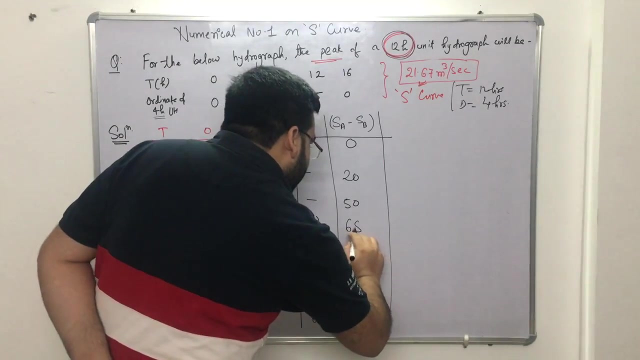 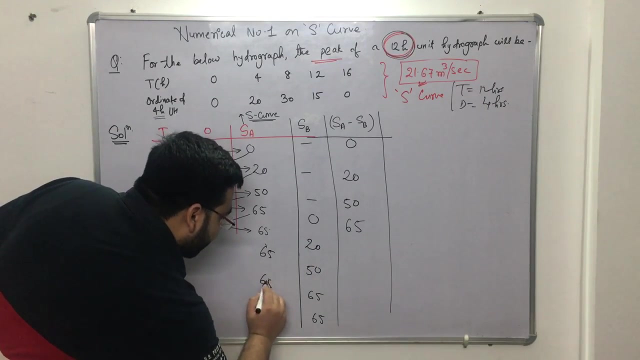 SB. this is the third step, right, This is 0,. SA minus SB is 0,. SA minus SB: 20, SA minus SB: 50, SA minus SB: 65, SA minus SB: how much Now? it will be equal to your. this will be 65, again 65, 65 and so on. so SA minus SB. 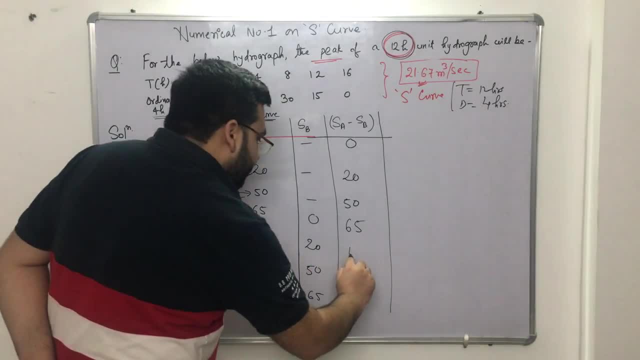 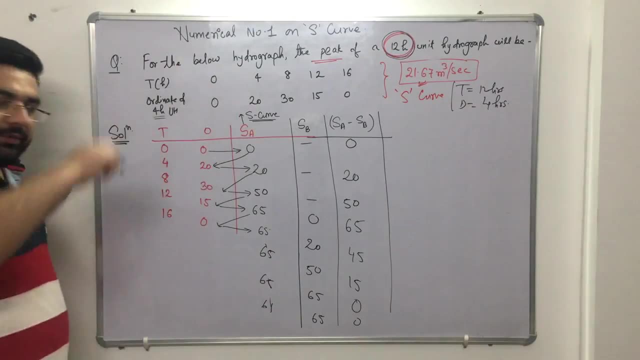 is 65, SA minus SB, it will be equal to 45, SA minus SB, it will be equal to 15, SA minus SB, it will be equal to 0, right, Right, Right. SA minus SB, it will be equal to 0, 0, 0, 0, 0, and so on, clear. 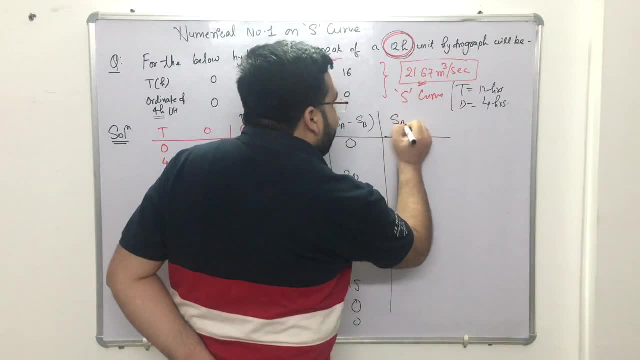 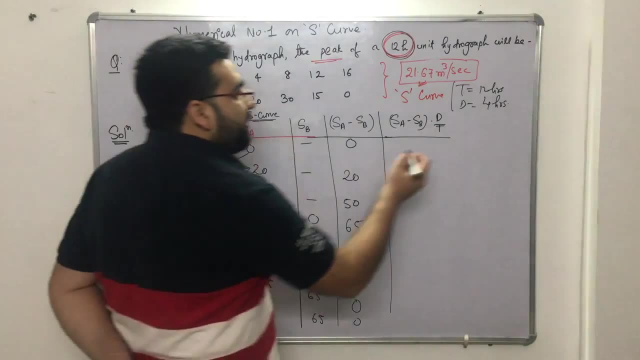 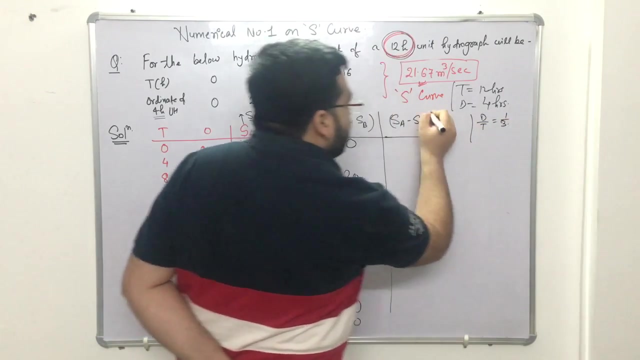 Now the next step would be SA minus SB into D by T, into D by T. Now, how much is D by T? So D is 4 and T is 12, so D by T will be equal to 4 by 12, that is 1 by 3.. 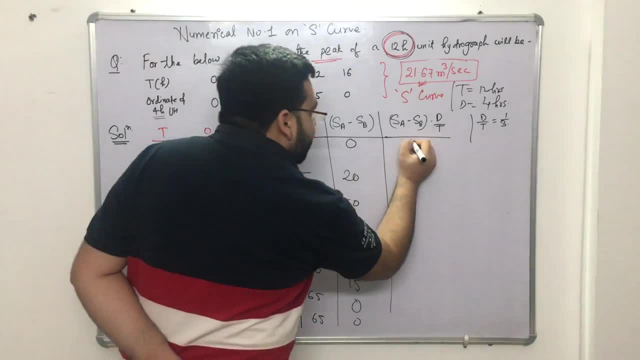 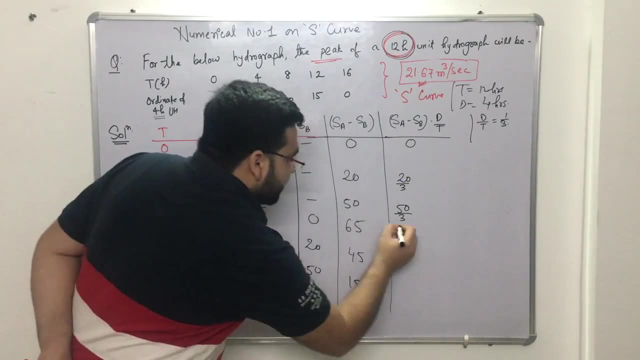 So I have to multiply it all by 3, right. So what will it be? It will be 0, 20 divided by 3, 20 divided by 3. Right, 50 divided by 3,. 65 divided by 3, right. 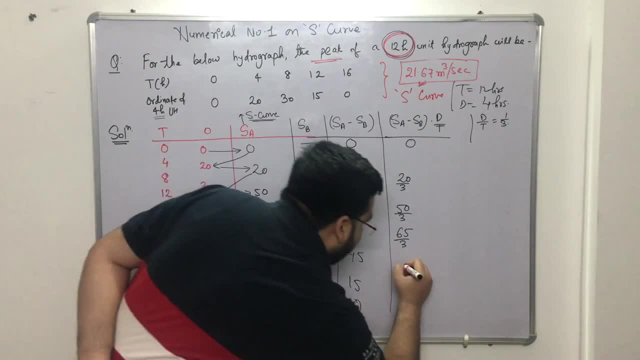 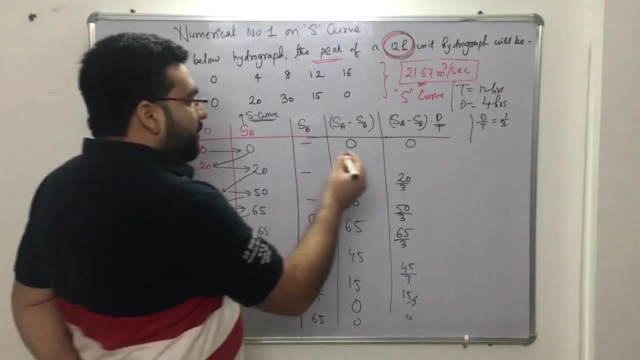 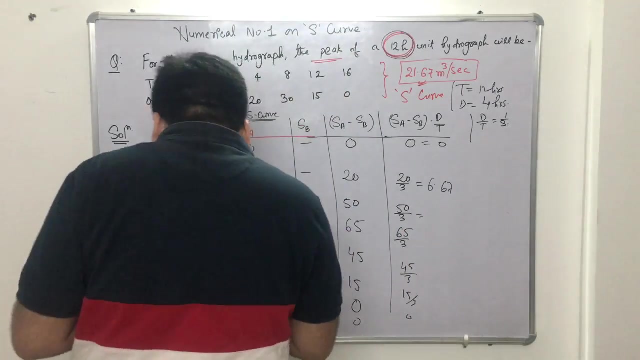 45 divided by 3,, 15 divided by 3, 0,, 0, 0 and so on. right, So how much it is? This is 0,. this is 6.67 something. So this will be equal to 50 by 3, let me calculate how much it is 50 by 3, exact value will: 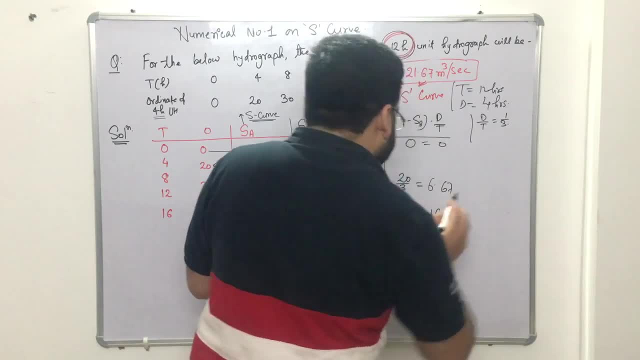 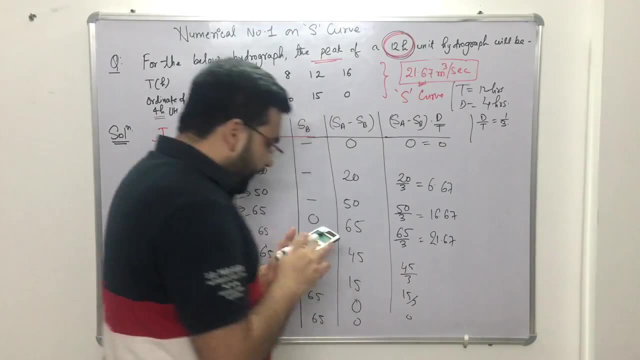 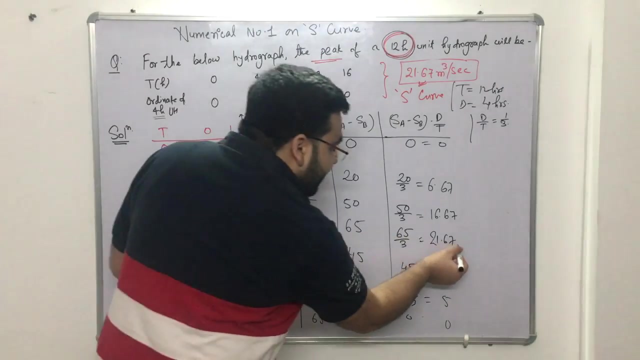 be 16.67.. 16.67,, 65 by 3,, 21.67,, 45 by 3,, 15 and 5 by 3, 5 and 0, right, So how much is the maximum value? 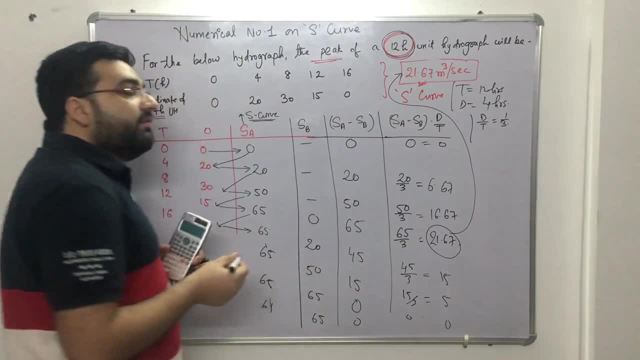 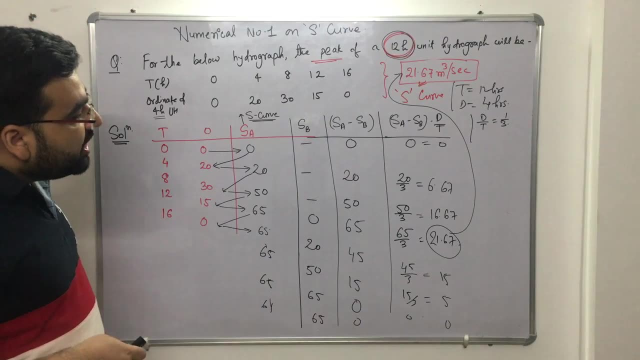 21.67 and the same answer we got when we solved this question with the method of superposition clear. So I hope that you have understood how to implement this method. Thank you, Bye, Bye, Bye, Bye, Bye, Bye. 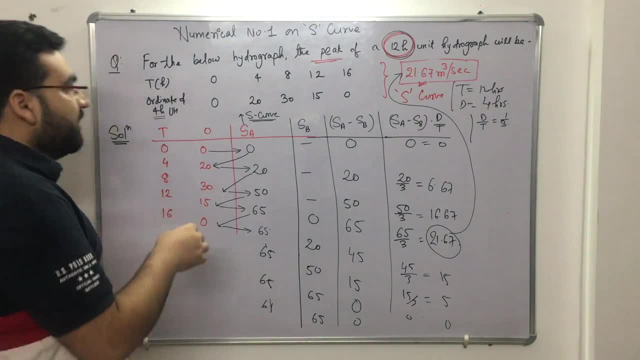 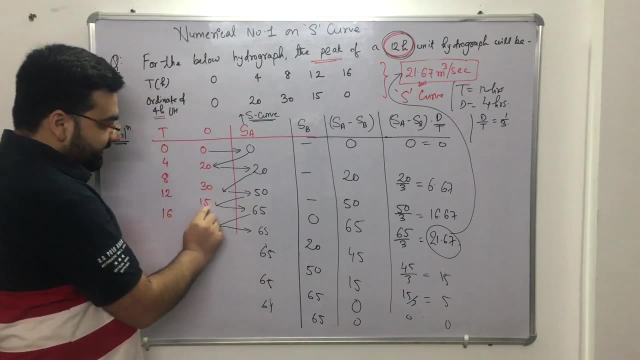 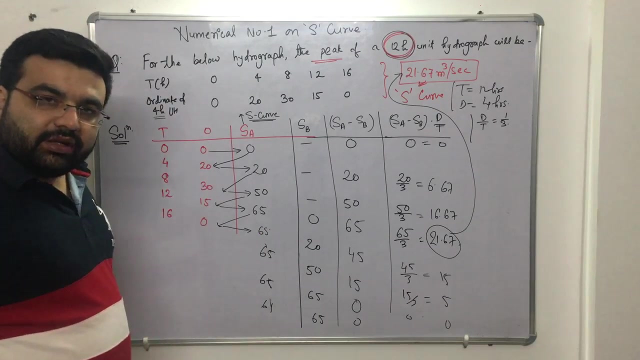 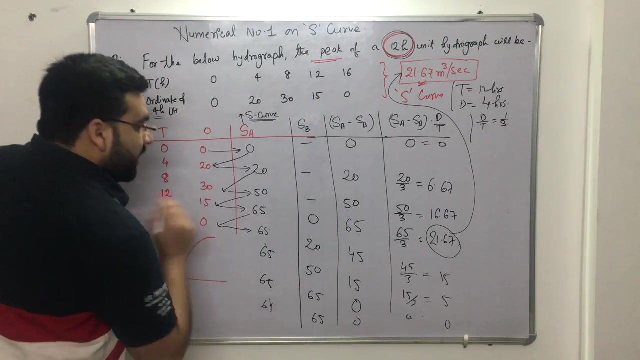 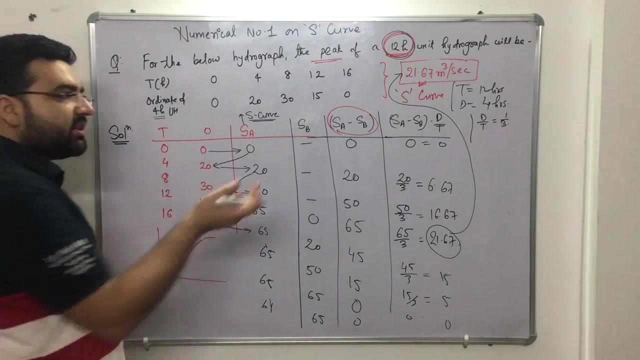 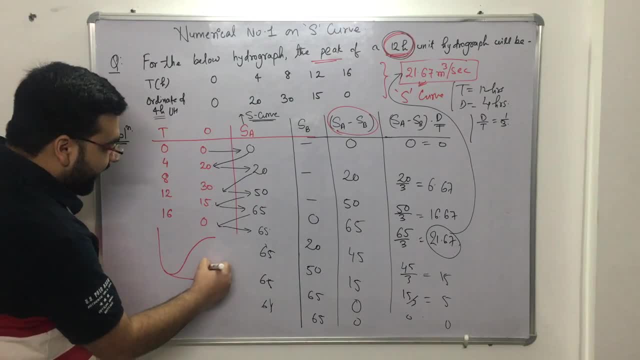 If in question 8 would have been asked, you would have lagged it by 8.. If 7, then by 7.. If 13, by 13, and so on. Okay, Now this is another S curve which is lagged by 12 hours. 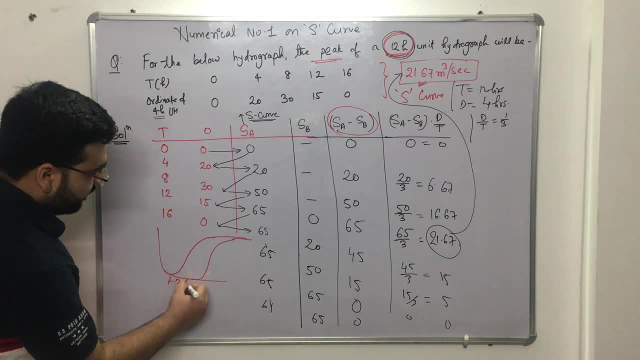 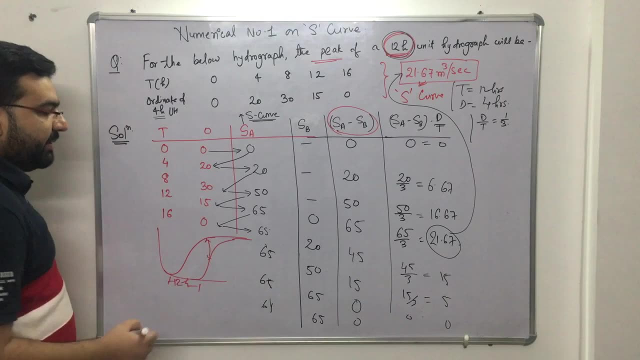 Another S curve, another S curve, it is lagged by 12 hours. Okay, Then what we have done? SA minus SB. Then we calculated SA minus SB and we multiplied S A 12 to 1.. Okay, 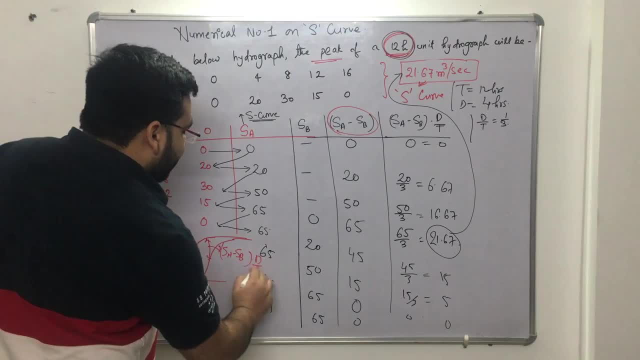 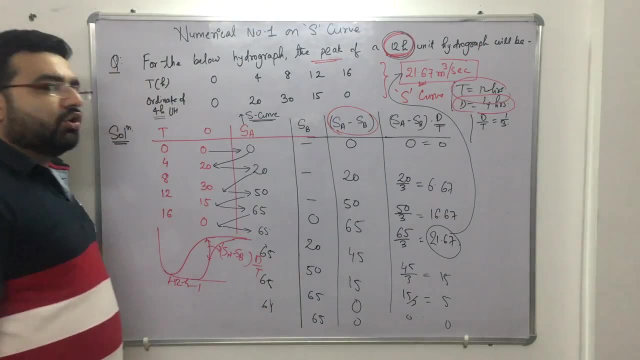 S A minus S B with D by T, How much is D? D is equals to your 4 R's, and how much is T? T is equals to your 12 R's. So D by T will be equal to 1 by 3.. 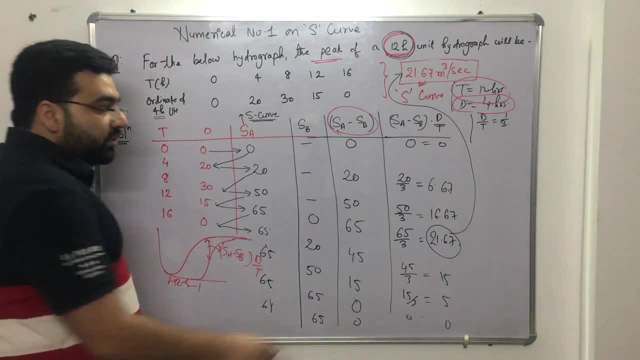 Or in other ways, we have to divide it by 3 and you will get the answer. So the same answer which we were getting from the method of superposition also, We have the same method. It is the same method, Okay. 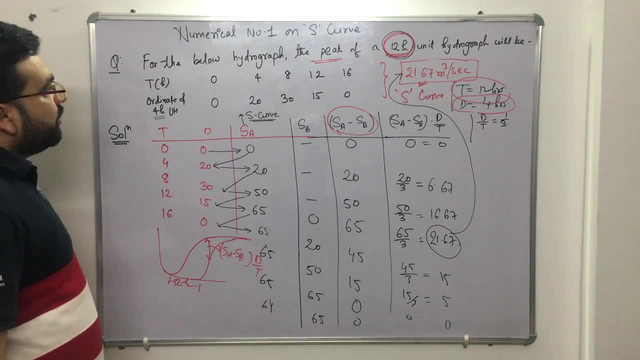 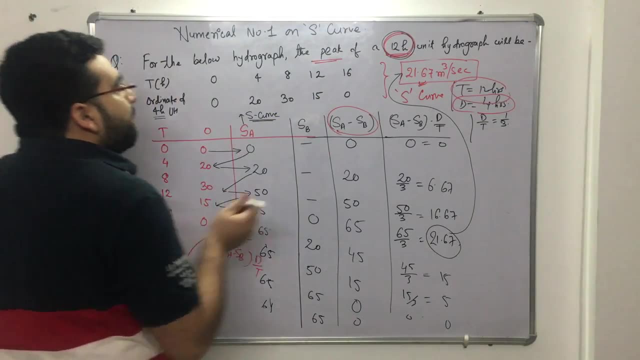 Now, sometimes the question can be like this. Sometimes the question can be like this: You are given a 4 R unit hydrograph and instead of this 12 R unit hydrograph, you are supposed to determine a 6 R unit hydrograph. 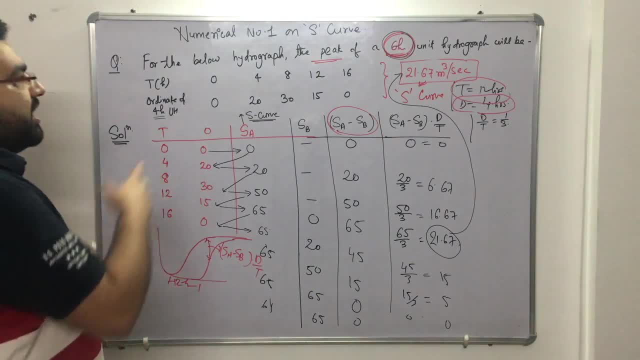 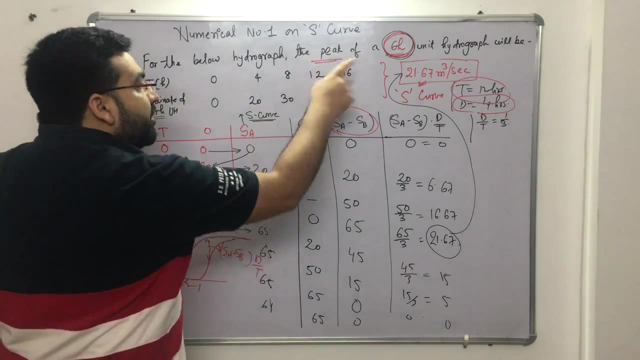 Let us say, For example- I am just taking an example- Let us say that you have to determine 6 R unit hydrograph. So first step would be similar, But on second step, what you have to do, You have to lag it with 6 R's. 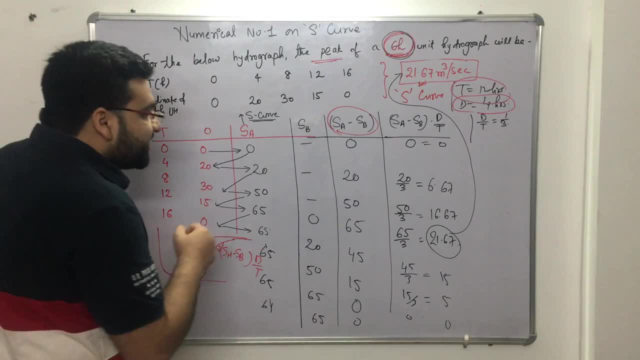 You have to lag it by 6 R's, Right? So how you can lag it by 6 R's? Because here you have 4, here you have 8. So 6.. 6 R's will be somewhere here. 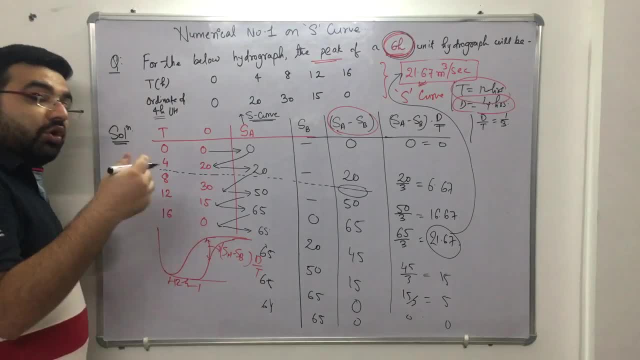 Will be somewhere here Here, But I don't know that. what is the value at 6 R's? Because I have to lag it by 6 R's At that time. what we do is that we break this 4 into smaller parts. 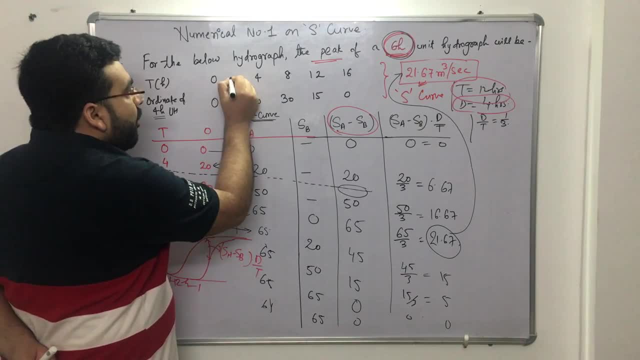 Let us say that from 0 to 20, it is 4. Right, Then I also take some 2, also Right. Take average of this: It is 10.. Right, It is 4 to 8.. Now 4 is 20.. 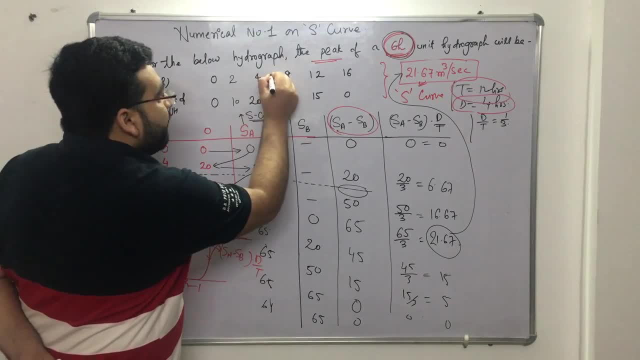 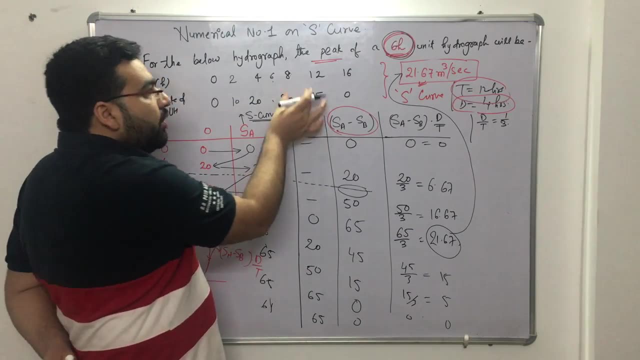 8 is 30. Then I will see how much is the incremental change. And for 6 also, I calculate the value. Then, for 8, it is 30.. For 12, it is 15.. I get the incremental value. 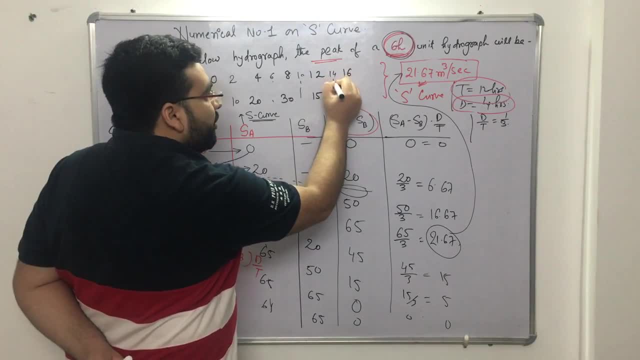 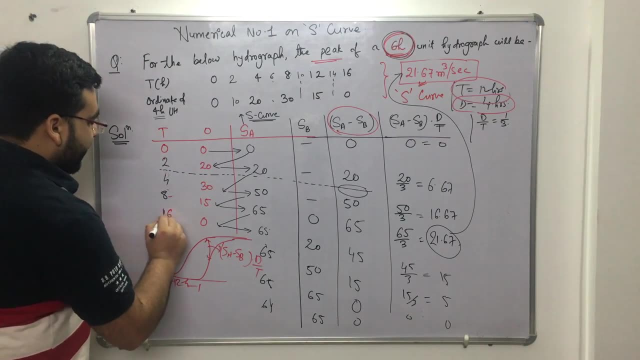 And I get the value of 10 also And similarly 14 also, Right. So this table I will draw for 0,, 2,, 4,, 8,, 10,, 12,, 16 and so on. 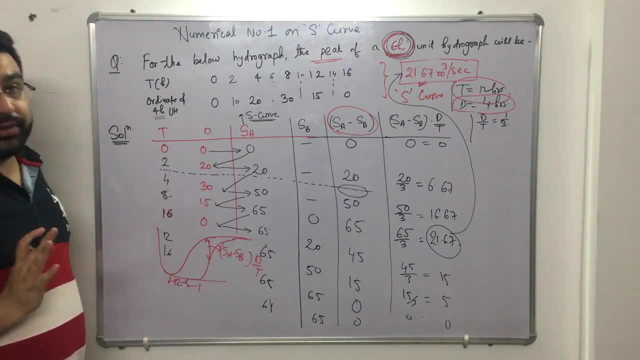 And that is how I can shift it with 6 R duration. Okay, So I hope that you have understood How to solve these types of questions with the help of S curve. Okay, Now let us move forward and understand a new topic which is generally asked in examinations.